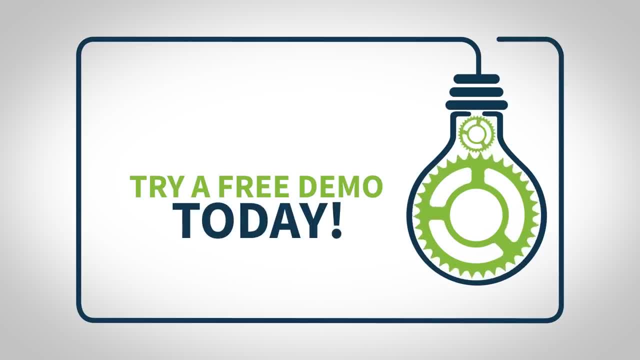 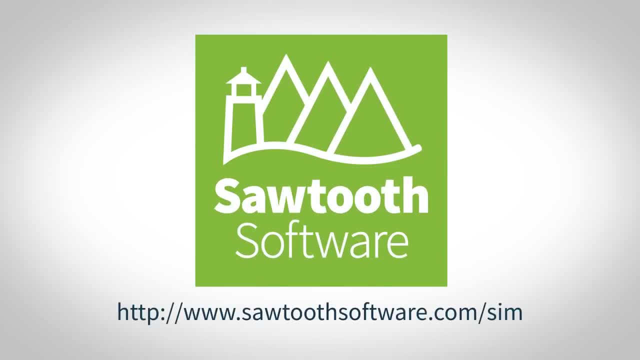 Try a free demo of the Choice Simulator today. To find out more, contact your research provider or visit us at saatusoftwarecom. Subtitles by the Amaraorg community. 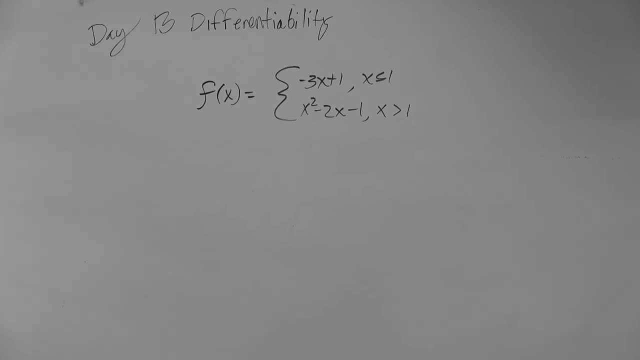 Would you guys agree? OK, So the first thing is, let's figure out where it's discontinuous. Now, both of these functions are continuous functions. Right? Both of these functions are continuous functions, So we know there's no discontinuity here. 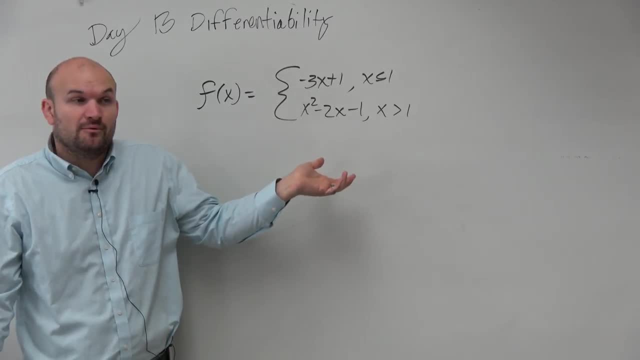 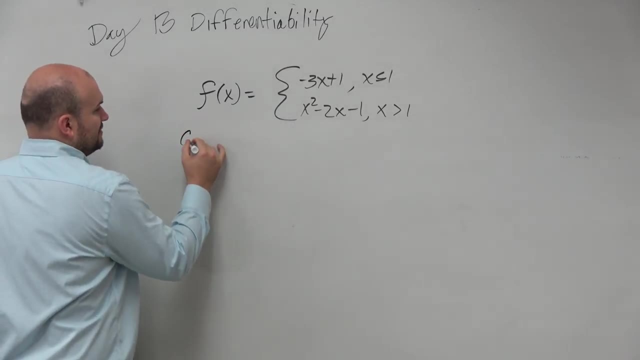 That's a line, That's a quadratic, But we know there could be a discontinuity. at what value? 1, right. So what we'd want to do is basically just check to make sure that the continuity- So I'm going to say negative- 3 times 1 plus 1. 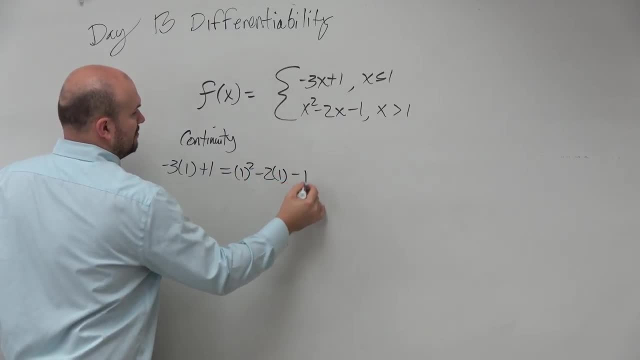 is equal to 1 squared minus 2 times 1 minus 1.. Therefore, I get here. it's going to be a negative 2.. This is going to be negative. 3 equals negative 2.. f of x is continuous. 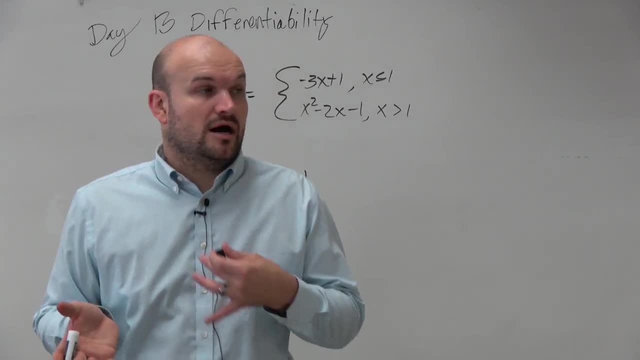 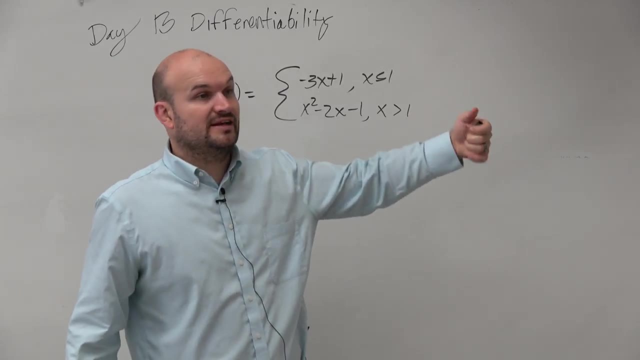 Make sense Continuous. That's good. Now we need to check. We need to check differentiability. So to make sure that this is continuous. what I wrote down is the derivative on: the left and the right have to be the same. 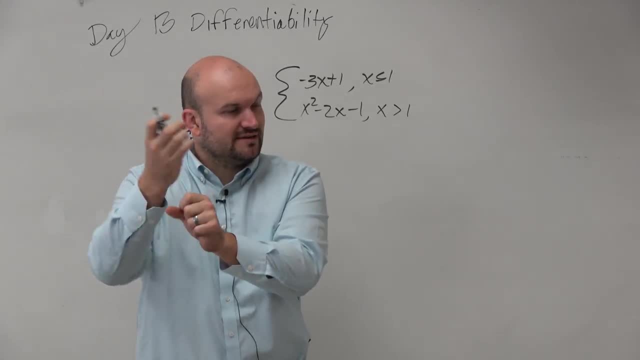 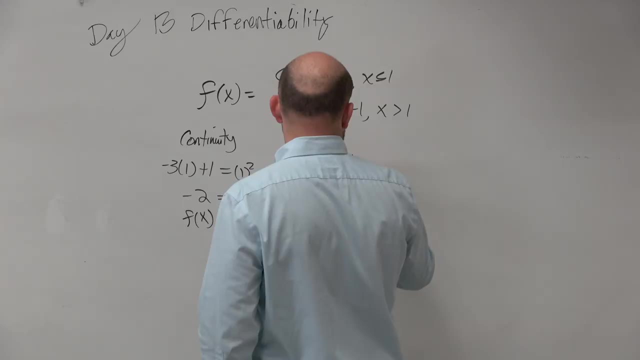 Right, You can't have two different derivatives, and then it's not differentiable. You have to have the derivative that's going to be equal on the left and the right hand side. So what we're going to do is now take the dr dx of negative 3x. 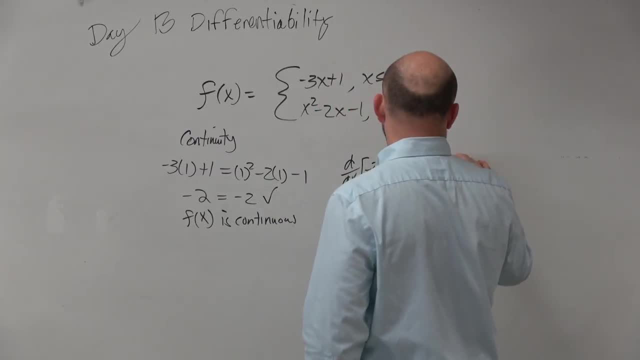 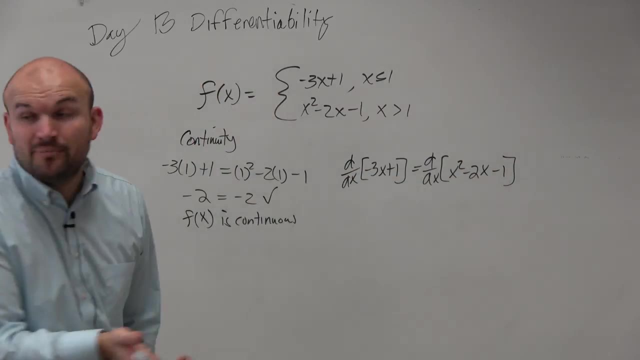 plus 1 has equal dr dx of x squared minus 2x minus 1.. OK, OK, OK, OK, OK, OK. And then at that point. So first thing, so that is at x equals 1.. This is at x equals 1.. 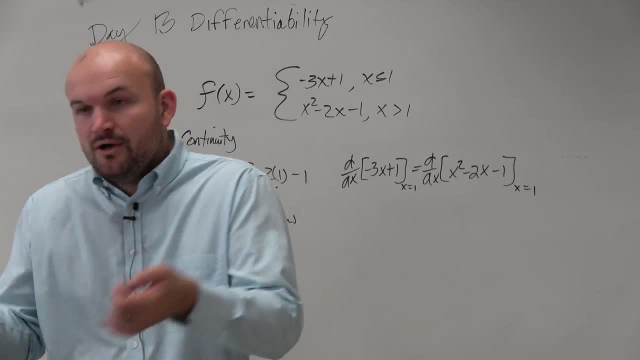 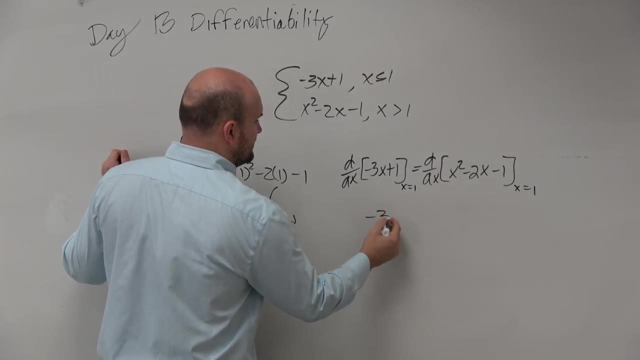 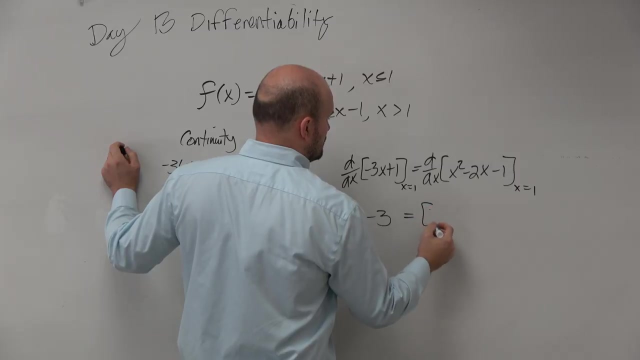 Right, We want to find the difference. The derivatives we know are not the same. We want to find: is the derivative the same at that point? So here we take the derivative which is negative 3.. Here we take the derivative which is going to be 2x minus 2..